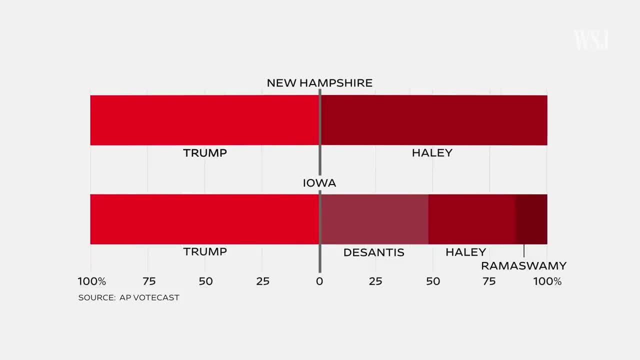 Trump voters on the left and the non-Trump voters on the right. In New Hampshire we're really talking about Haley voters In Iowa. we'll do a weighted average of the voters who voted for her, DeSantis or Ramaswamy. 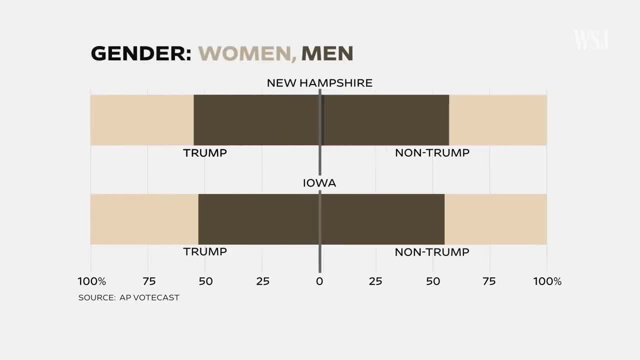 If you look at some of their basic demographics, the difference doesn't lie in gender. Both the Trump and non-Trump voters have about equal amounts of men and women. It doesn't lie in age either. They are equally people with guns in their homes and just as likely to be evangelical Christian. 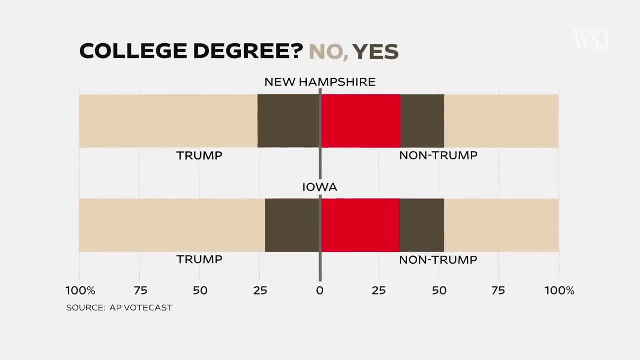 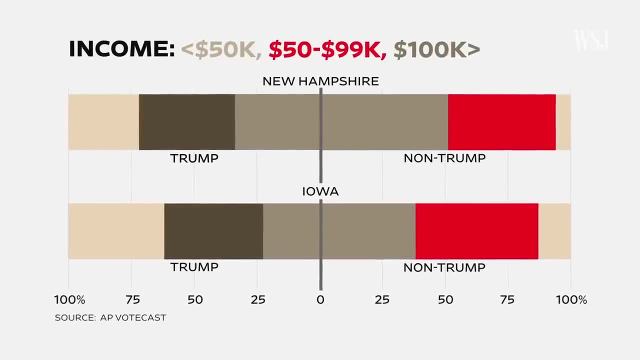 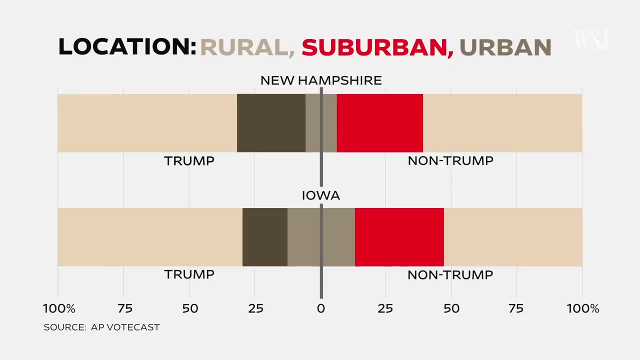 But differences come up when you look at education. Non-Trump voters are more likely to have college degrees And at income. Most earn above $50,000. Or even $100,000. And they tend to be more suburban, just like the Republican Party was before Donald Trump. 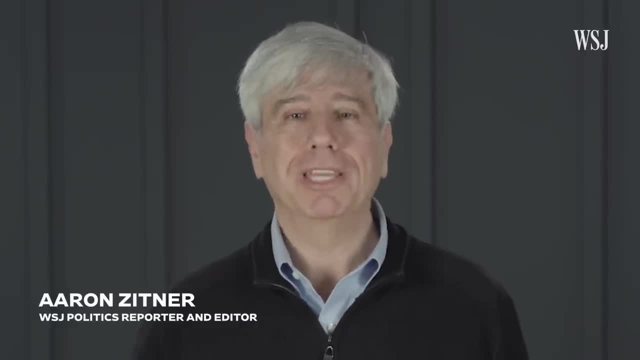 We used to have a kind of voter we called the country club, Republican, Upper income and suburban. Donald Trump activated people who didn't vote very much before. We know that he's brought in a lot of working class people, But in the course of doing that he's alienated others. 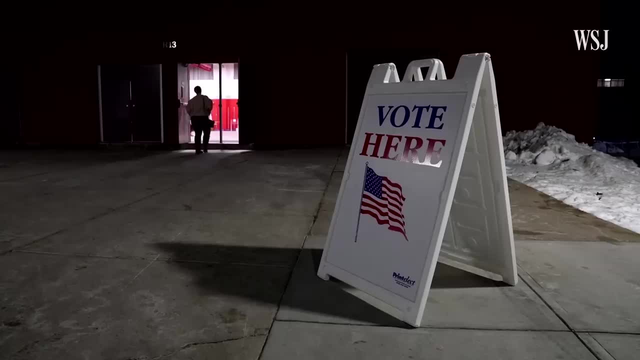 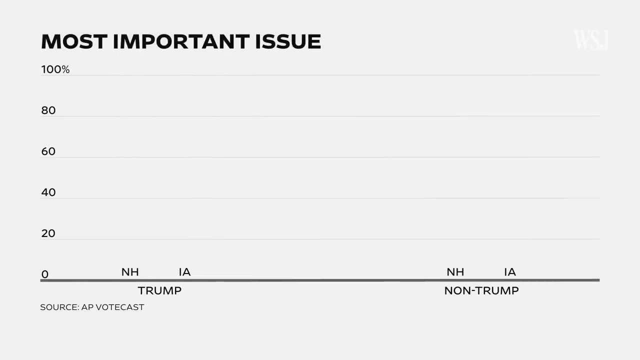 So what we're seeing in those states is who he's pushing away. To see who that is, there are two things. One, the issues they care about. Trump and non-Trump voters equally care about the economy, But non-Trump voters care less about immigration. 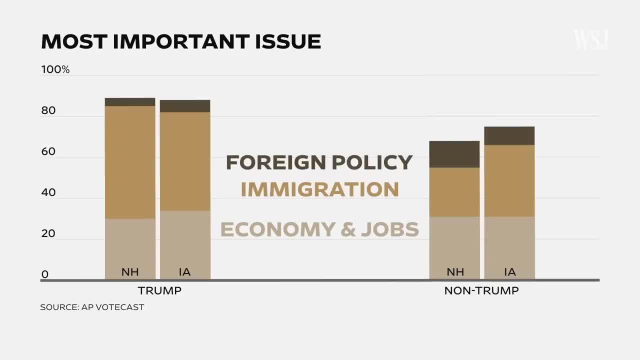 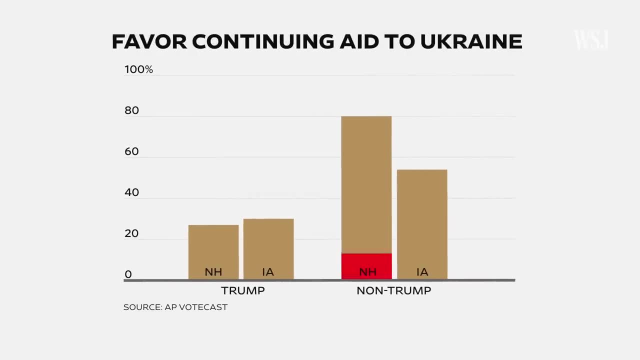 And two times more about foreign policy. They also care more about domestic issues like abortion and healthcare. Non-Trump voters also favor continuing aid to Ukraine, especially in New Hampshire, where more independent voters wait in. But more than half of Trump voters say that it's important to them to have a Republican nominee, and not just one. 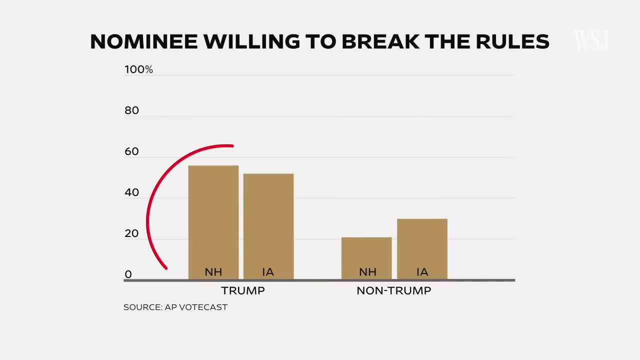 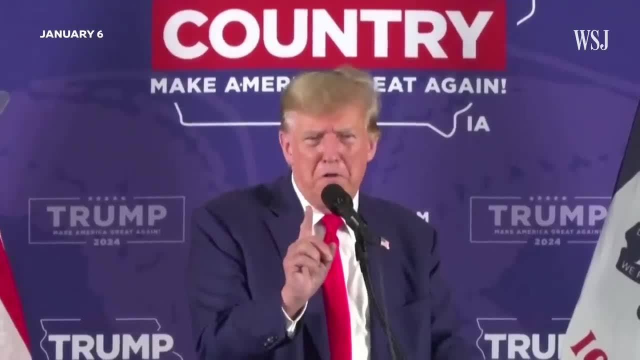 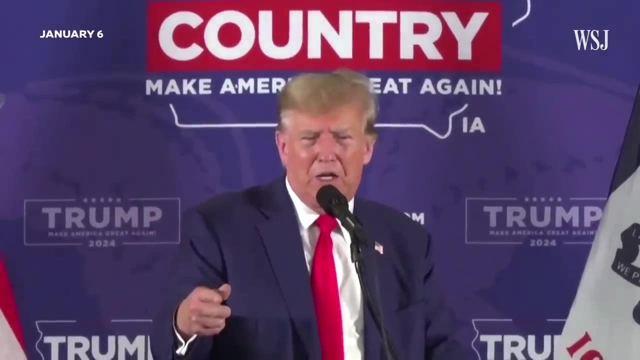 Trump himself is a Republican nominee that's willing to break the rules to get things done, Which hints at the larger theme separating these voters: Trump himself. I'm going to be a dictator for one day, For drilling and for closing the border, And after that I'm not going to be a dictator. 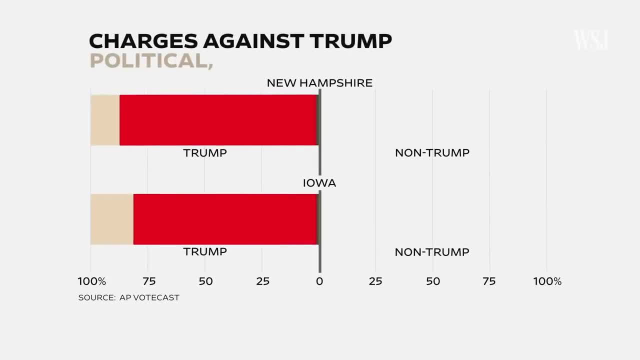 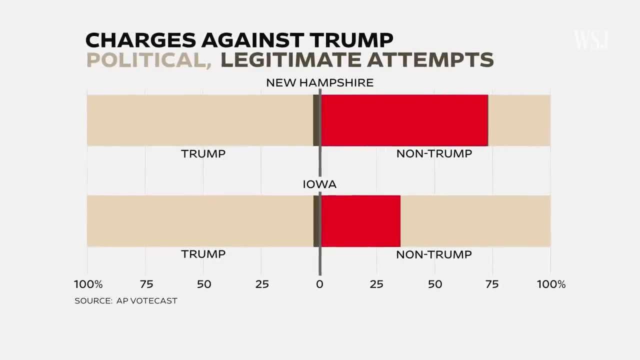 When asked about the charges against Trump, nearly all of his voters described them as political attempts to undermine him, While non-Trump voters were more likely to describe them as legitimate attempts to investigate important issues. It's a witch hunt in the truest sense of the word.